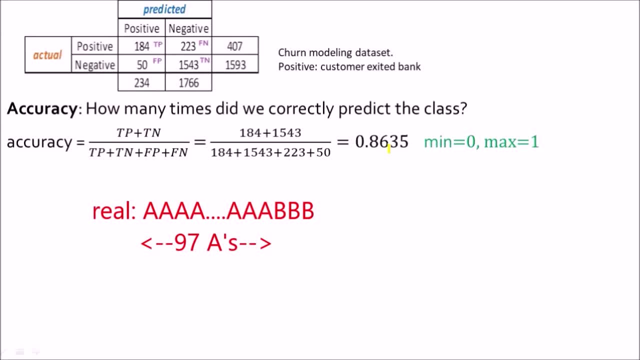 Then even if I make a classifier that predicts class A every single time, even then I would be left with a 97% accuracy, Because there are 97 class A labels, right? Even a 97% accuracy doesn't look good. Even a 97% accuracy doesn't look very good in that sense. 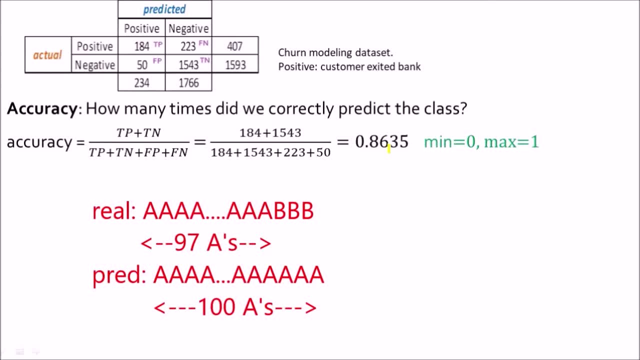 Hence, accuracy is not a very good measure when we are dealing with an imbalanced dataset. Next is precision. Precision is telling us out of all the times that we predicted positive. how many times were we correct? Well, so, how many times did we predict positive? 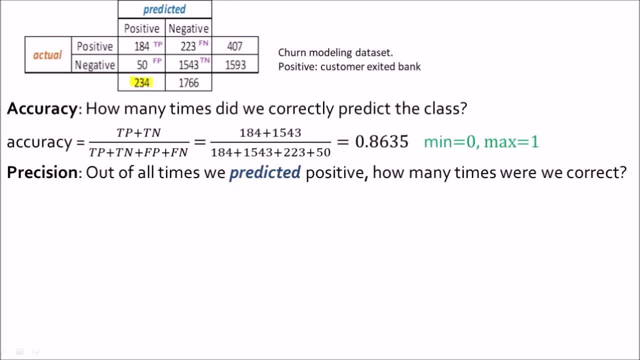 So, as we see here, 234 times we predicted positive. So, out of all of these 234 times, how many times were we correct? 184 times we were correct Because 184 times we said correct. We said the person will leave the bank and it was also the case in reality. 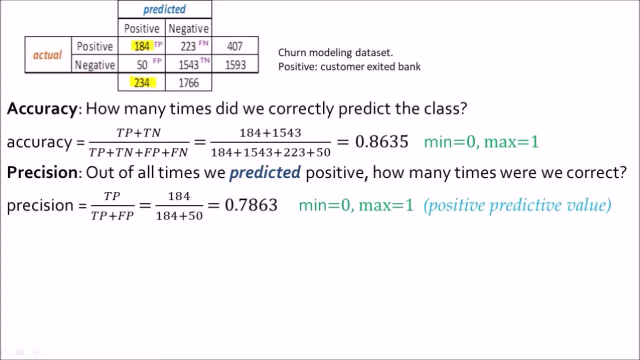 Hence precision becomes 184 divided by 234, which is 78%, And precision is also called positive predictive value. Basically, we are answering the question of how precise were the classifier's predictions of the positive class. So by default, when we talk about precision, recall F1 score etc. 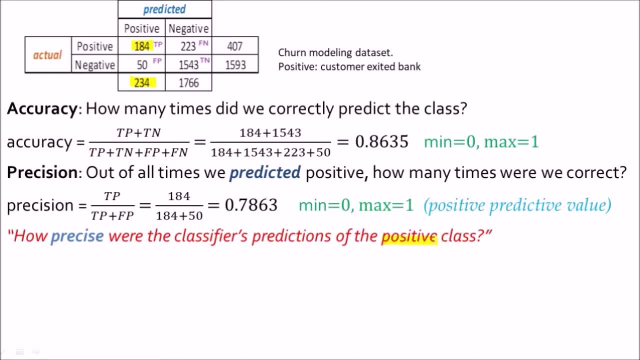 We talk about the positive class only. Okay, So we have the positive class and we are deriving these metrics by default or by convention. Next is recall. Recall is out of all the times that the real class was positive. How many times were we correct? 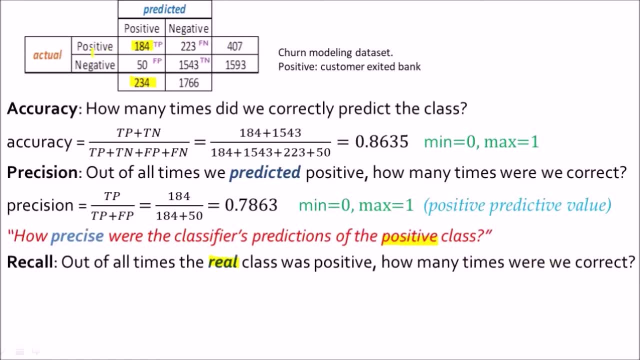 So how many times was the real class positive? Well, we see actual positive and we look at this: 407 times The actual class was positive. So in reality, in the test set there were 407 people that really left the bank. 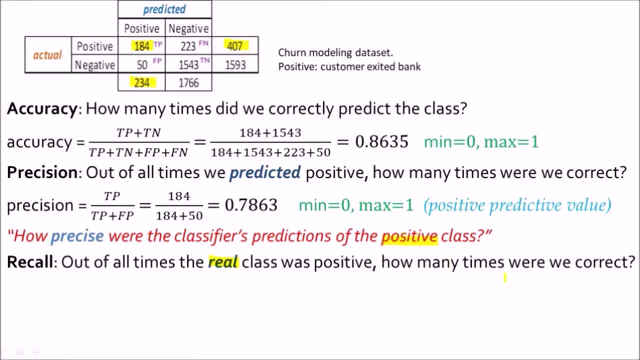 And out of all those 407 times, how many times were we correct? Well, again, 184 times we were correct and 223 times we were incorrect. So our recall becomes 184 divided by 184 plus 223, which is 45%. 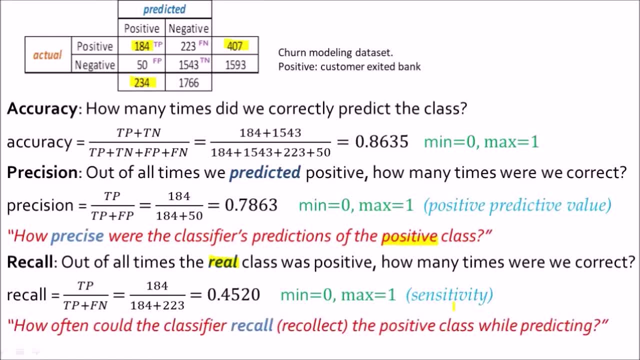 And recall is also called sensitivity. Now, when we talk about recall, we are basically answering the question: how often could the classifier recall or recollect? recollect, which is a standard English word, the positive class while predicting. So how many times was it able to recollect, as in